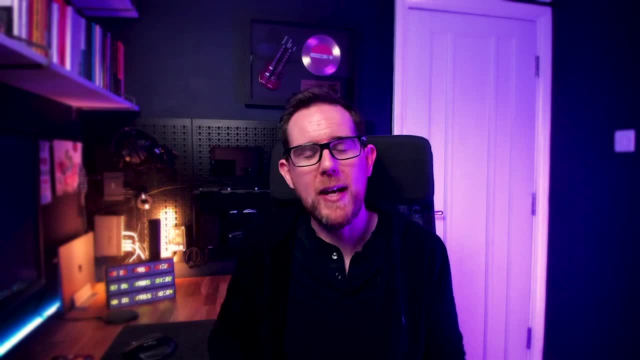 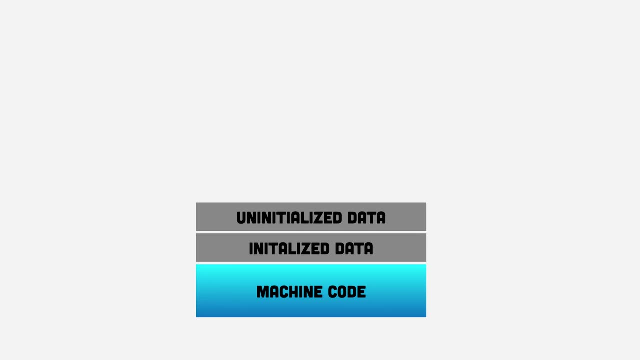 to work out why things have different scopes. Now the memory of your application is stored in three main parts. The first part is the machine code. This is where your application is converted into instructions that your computer can understand. The next two parts are the stack and the heap. 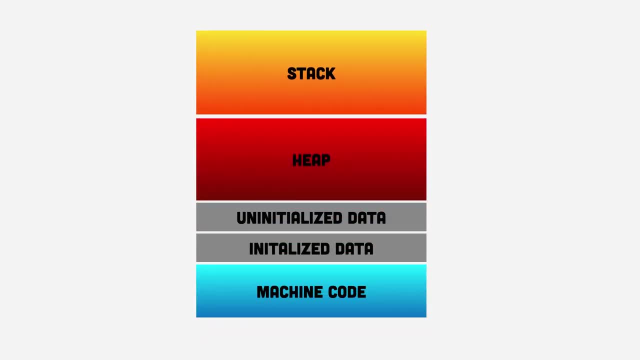 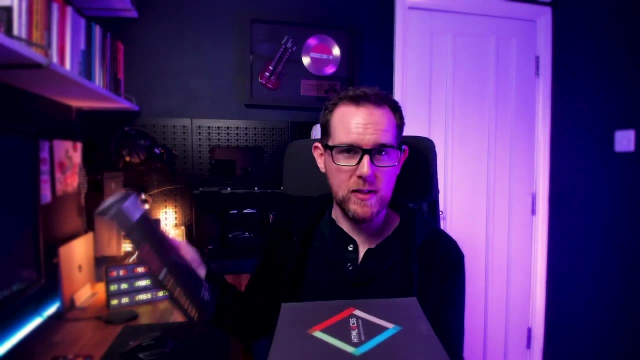 Now, to understand the stack, you need to understand the stack data structure. Now, the stack data structure is a little bit like a stack of books, So you can imagine you've got a book stacked like this: You can take things off the top of the stack and you can put things on the top of the stack. but 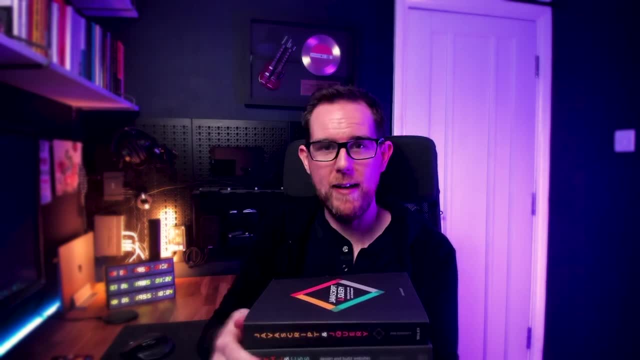 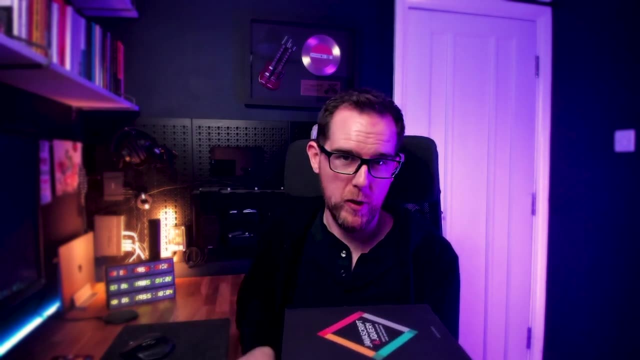 you can't access anything with the remainder of the stack. So we can't take anything from the middle, we can't take anything from the bottom. All we can do is just add stuff to the top, take it off, and in that order. Now in applications we have what we call the call stack, Now the call. 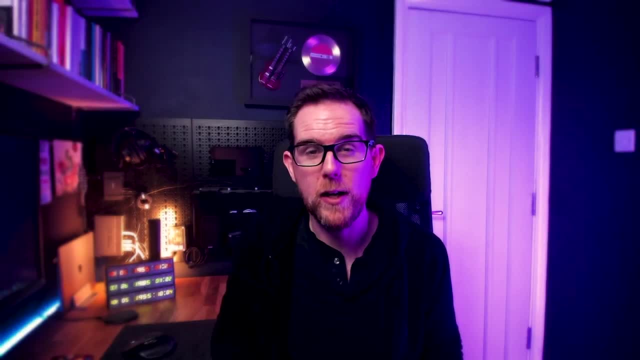 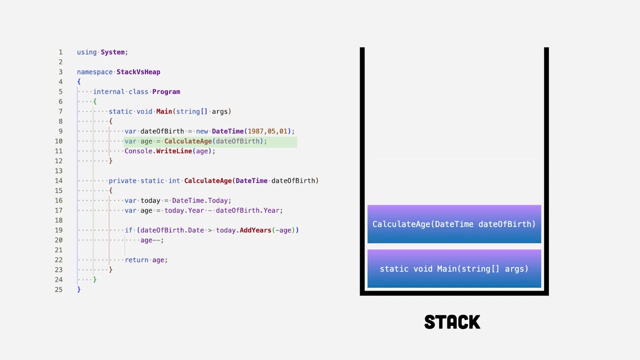 stack has a couple of responsibilities. The first is to keep track of the method that control should be returned to after the current method is finished executing. So whenever you call a method in your code, that's going to get added to the call stack and each. 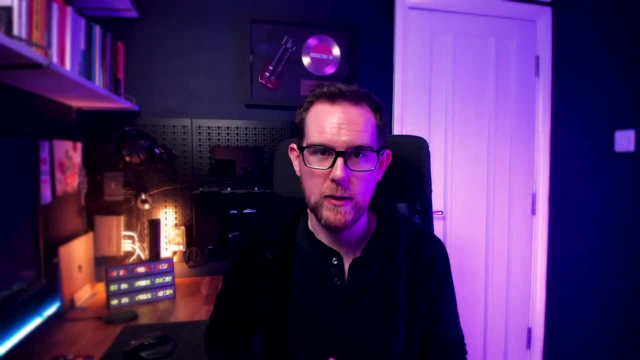 subsequent method is just going to get added to the call stack until they finish executing. Now the second thing that the call stack is responsible for is for keeping track of the local variables in your method. In a minute I'll also be covering where the other variables are. 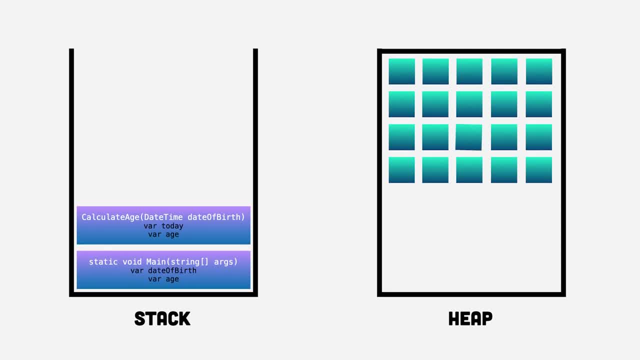 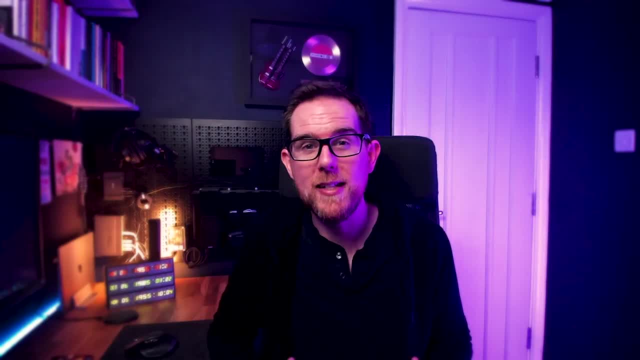 stored in memory. Now the heap, unlike the stack, allows you to store items in memory in any order. You're not limited to take this top item from the stack. you can access it from anywhere. Now, with this added ability, it becomes a bit more complicated when it comes to adding and removing. 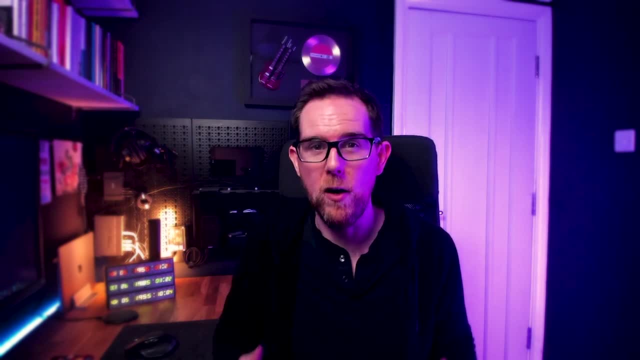 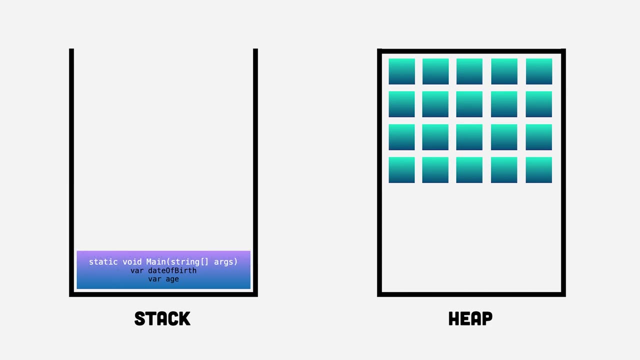 items and therefore adding items to the heap has a higher overhead than it does adding items to the stack. Now, generally, the heap is used whenever you have data that's going to outlive what's on the call stack. So if you have a variable that needs to be accessed across different methods, 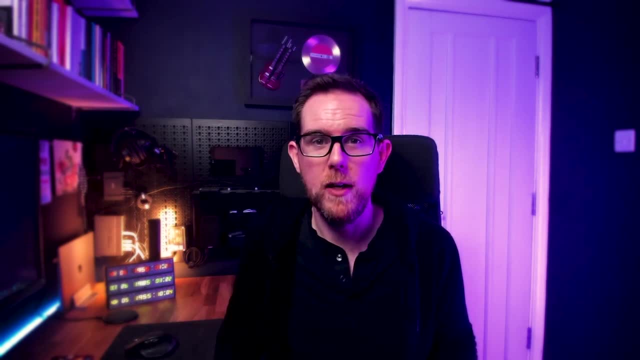 or some data that needs to be accessible after a method is run, then that is going to live on the heap. Now there are some general rules that you can apply to work out where your variables are going to get stored in memory. In a previous video I talked about how we have value type. 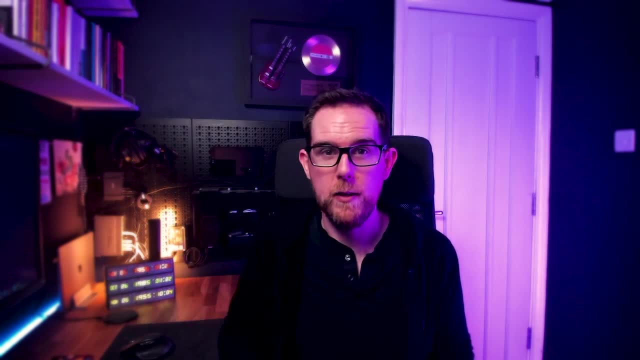 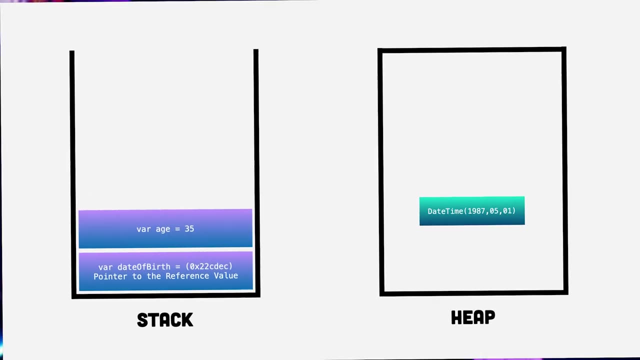 and reference types. Now, value types just store the value. So generally, data types such as this, such as int, will be stored just as a single value in memory, Whereas a reference type has a pointer to a value. So we have two parts to a reference type. We have a pointer, which is generally just: 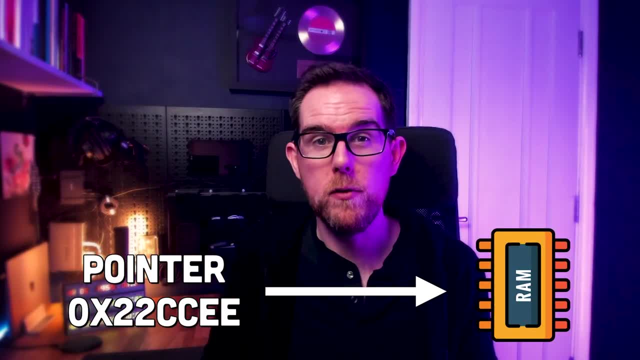 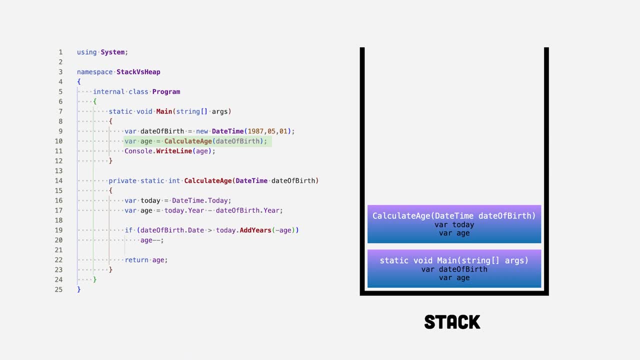 an address to a location in memory. Now, the values for reference types are always stored on the heap For value types. it really depends on where you declare it. Now, when you create a local variable in a method, we know that we can't access that variable from outside the method and the 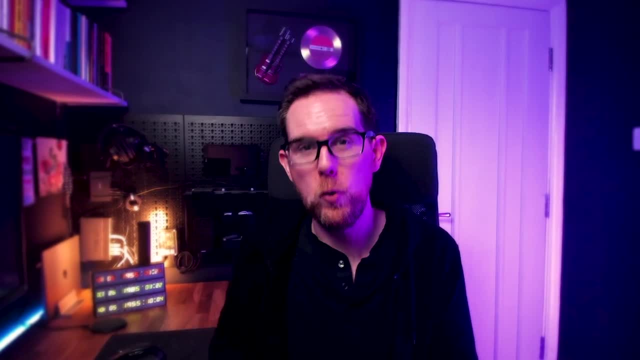 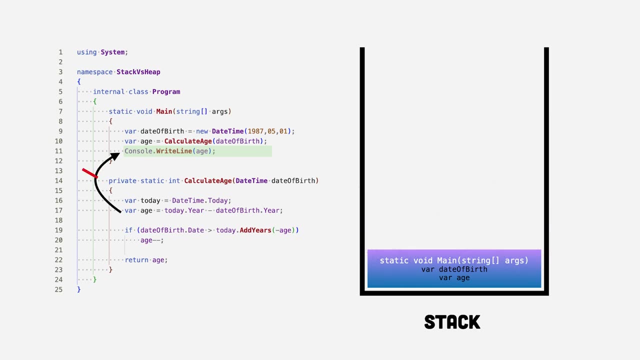 reason for that is because that local variable is going to get stored on the call stack with the method. So as soon as execution is finished, that block on the call stack is going to drop off and therefore that local variable isn't going to be available anymore. Now if we were to declare a 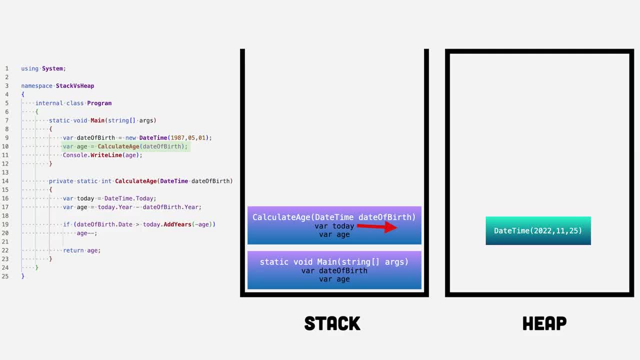 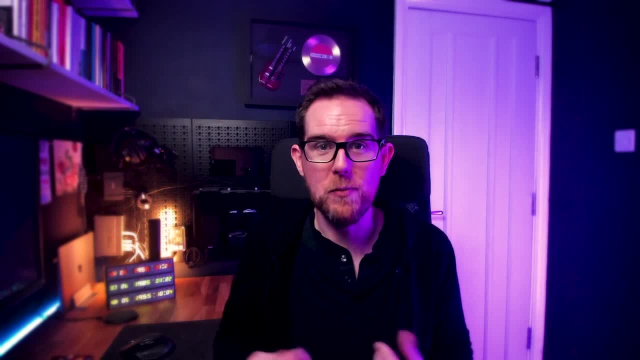 reference type variable inside your method, then it's just the pointer that stays on the call stack. The value for your reference type variable will be on the heap, but of course you can't access it because the pointer itself is gone once the method execution is finished. Now not all value types get. 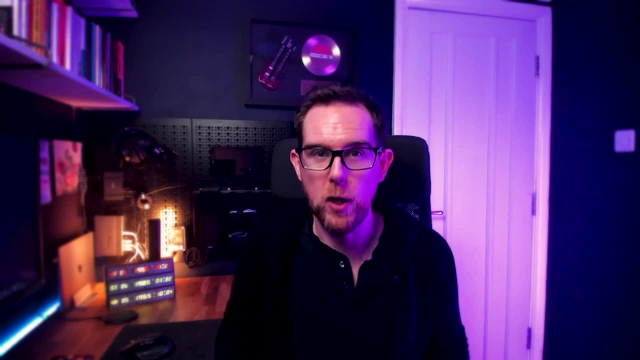 stored on the stack. If you have a reference type variable that is stored on the call stack, then you really depends on where you declare it in your code. So if you have a global variable, then that's always going to be on the heap because you need to be able to access it from different areas in your 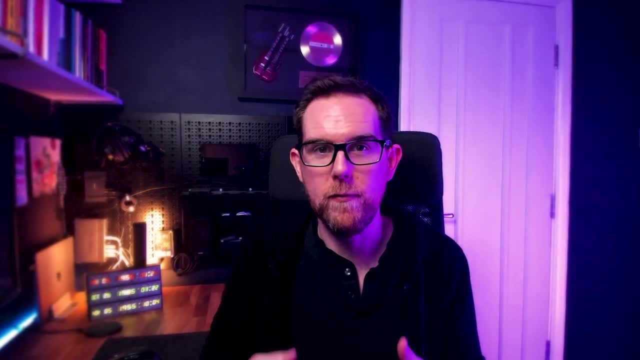 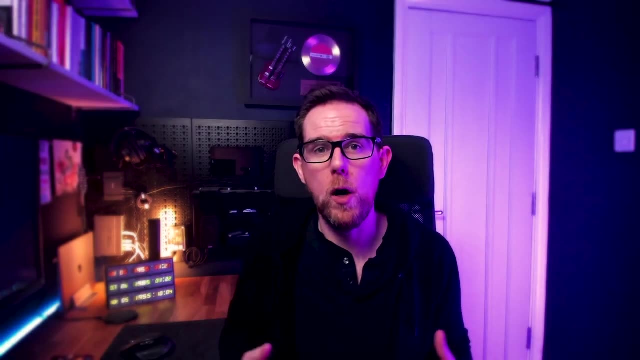 code. And, for example, if you create a class and then have variables inside your class and therefore that class is also going to live on the heap and so are the variables inside it, Now, because our reference types only have a pointer to location in memory, you have to wonder what happens to that. 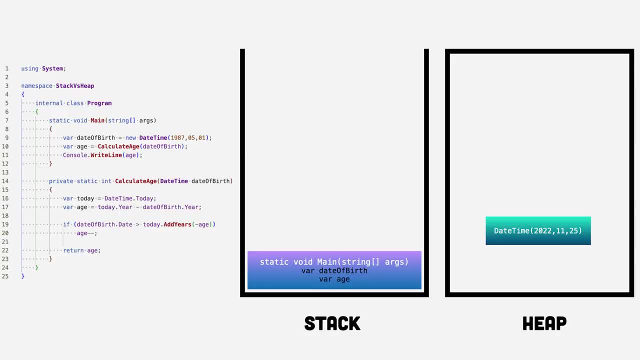 block of memory after your method is finished executing. In most runtimes we have what we call a garbage collector. The name suggests: a garbage collector goes around collecting garbage. It goes around and looks at the heap and finds things that aren't being used anymore and clears them up. So 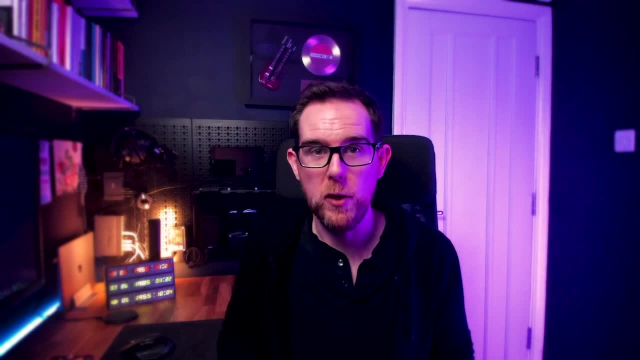 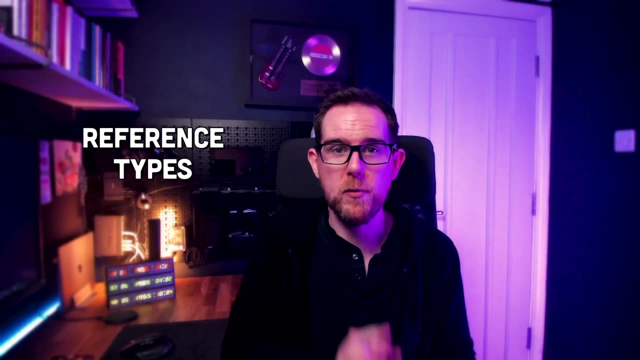 this is how, when a reference type that's declared in a method is no longer used, the pointer goes, and then, because there's nothing pointing to it, the garbage collector comes and cleans it up. So they're the general rules. You've got reference types always on the heap. Value types are either: 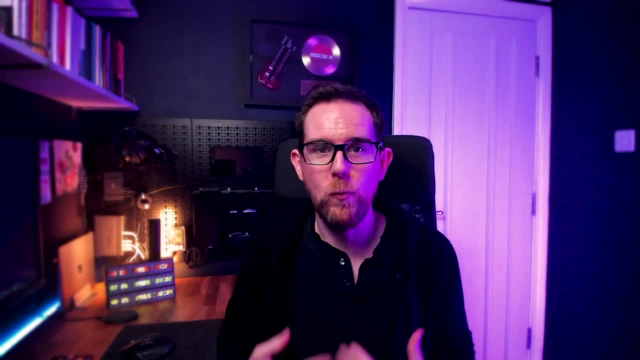 on the stack or the heap, depending on where they're declared. Now, of course, with all things, there are a few exceptions. Static variables, for example, will always be on the heap, Because you need to be able to access them from anywhere in your code. Now, in some languages, such 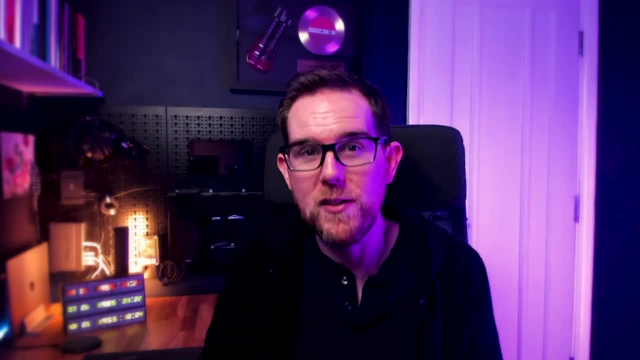 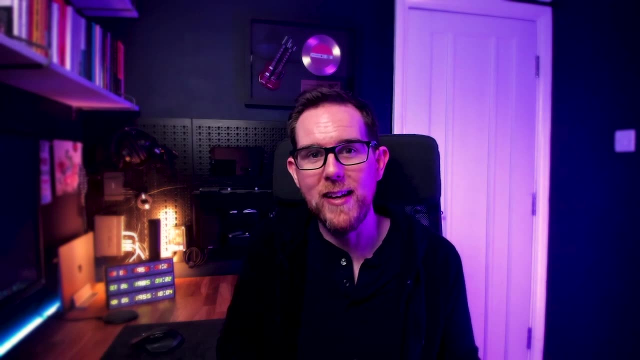 as C sharp, we have what we call anonymous functions. Now, as the name suggests, they don't have a name, but they can be created and called from inside another method. Now the thing with anonymous functions is that they have access to the other variables that you declared in the method. that